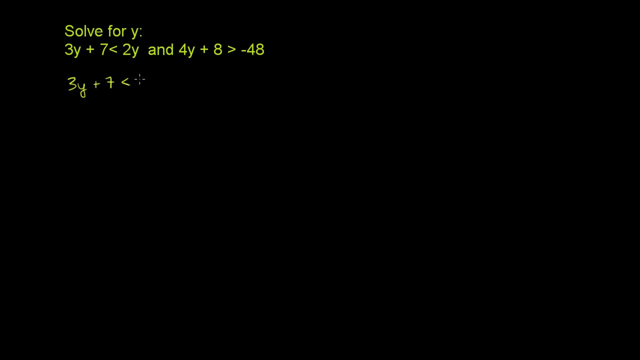 So we have 3y plus 7 is less than 2y. So let's isolate the y's on the left-hand side, So let's get rid of this 2y on the right-hand side, And we can do that by subtracting 2y from both sides. 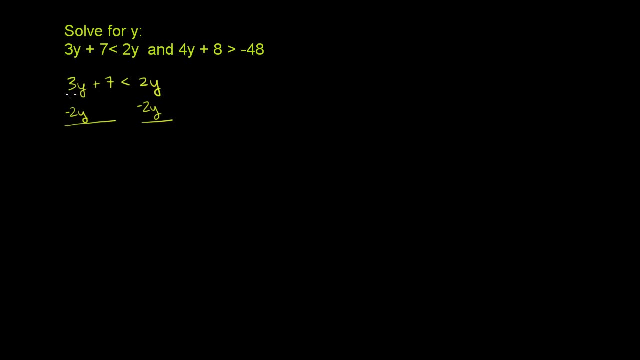 So we're going to subtract 2y from both sides- The left-hand side- we have 3y minus 2y, which is just y plus 7 is less than 2y minus 2y, and there's nothing else there. That's just going to be 0.. 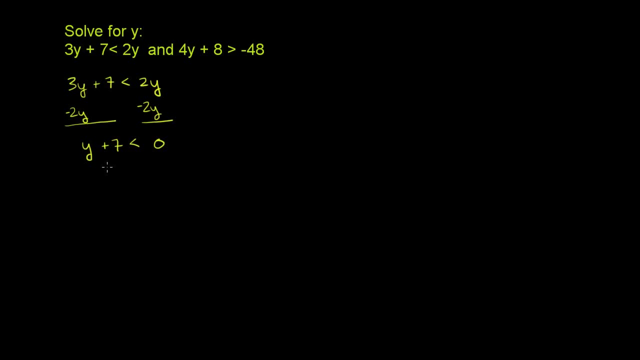 And then we can get rid of this 7 here by subtracting 7 from both sides. So let's subtract 7 from both sides. Left-hand side: y plus 7 minus 7.. Those cancel out. we just have a y is less than 0 minus 7, which is negative 7.. 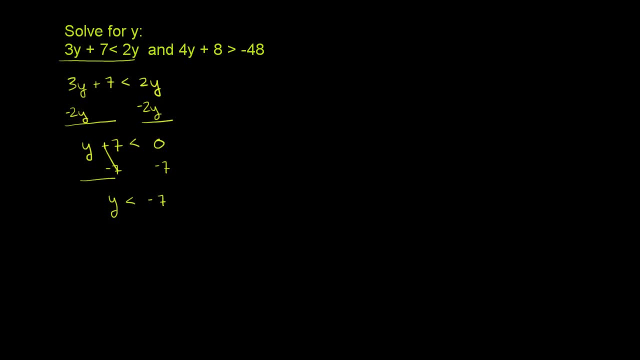 So that's one of the constraints. That's this constraint right over here. Now let's work on this constraint. We have: 4y plus 8 is greater than negative 48. So let's get rid of the 8 from the left-hand side. 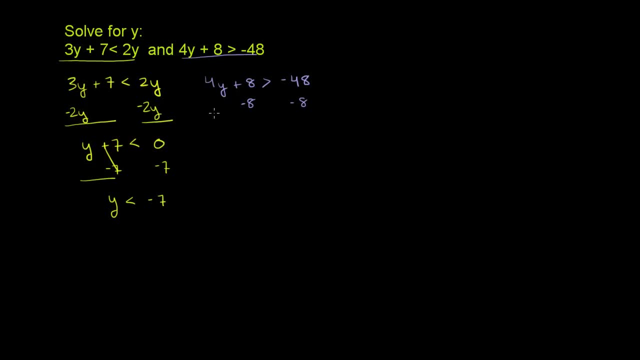 So we can subtract 8 from both sides. Subtract 8 from both sides- The left-hand side- we're just left with a 4y. because these guys cancel out. 4y is greater than negative 48 minus 8.. 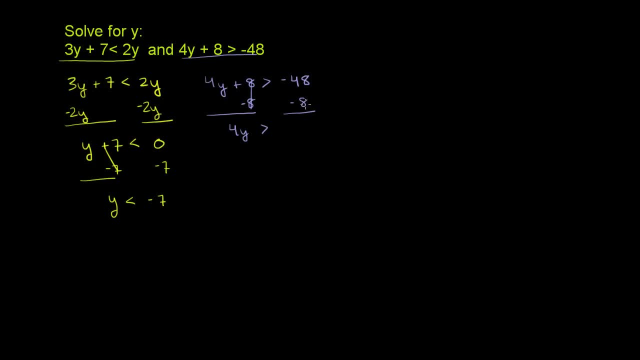 We're going to go another 8 negative. So 48 plus 8 would be 56. So this is going to be negative 56, negative 56. And now to isolate the y, we can divide both sides by positive 4.. 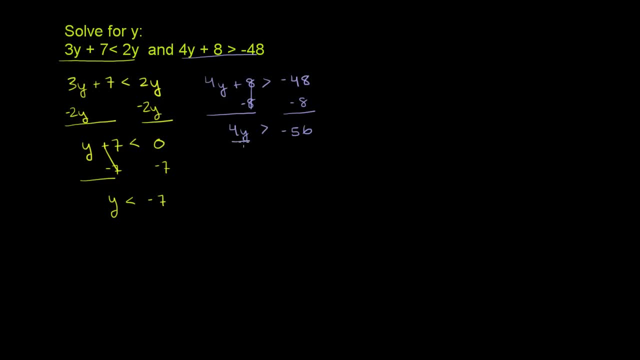 And we don't have to swap the inequality, since we're dividing by a positive number. So let's divide both sides by 4 over here. So we get y. We get y is greater than what is 56 over 4, negative 56 over 4?. 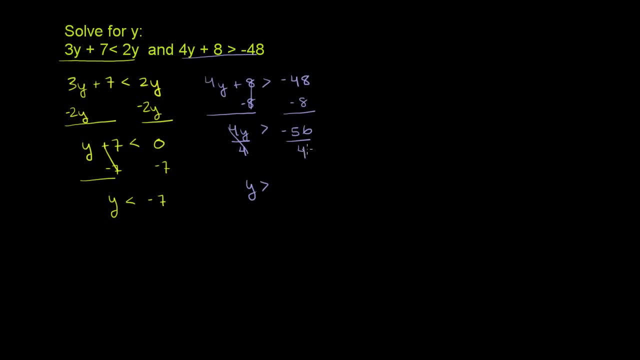 Let's see: 40 is 10 times 4, and then we have another 16 to worry about, So it's 14 times 4.. So y is greater than negative 14.. Is that right? 4 times 10 is 40.. 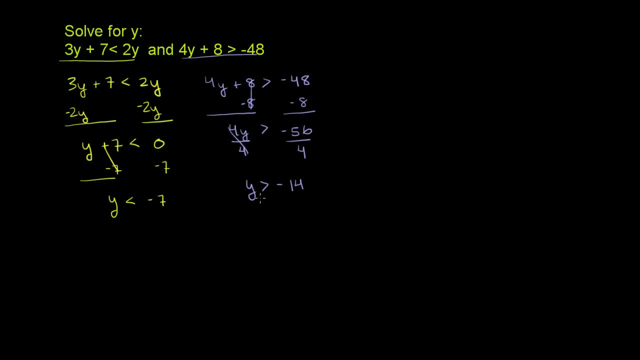 4 times 4 is 16.. Yep 56. So y is greater than negative 14, and let's remember we have this and here and y is less than negative 7.. So we have to meet both of these constraints over here. 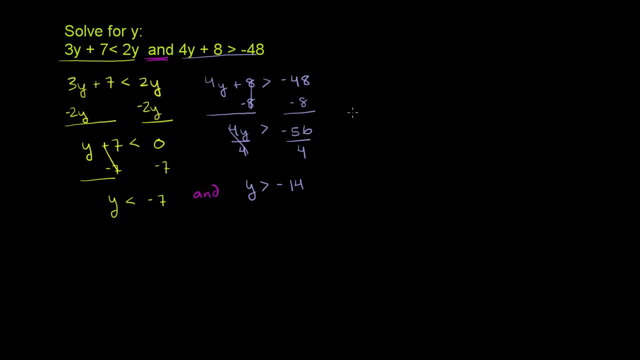 So let's draw them on the number line. So I have my number line over here And let's say: negative 14 is over here, Negative 14, so you have negative 13,, 12,, 11,, 10,, 9,, 8,, 7.. 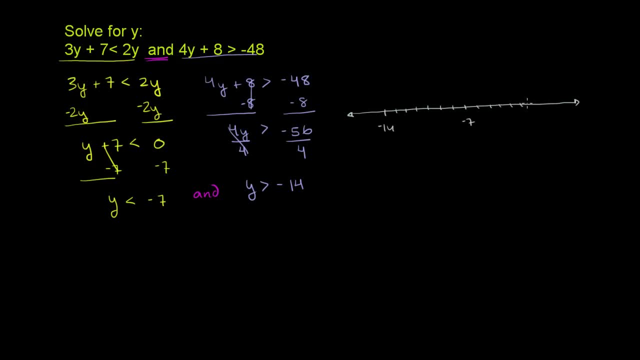 That's negative 7.. And then negative 6,, 5,, 4,, 3,, 2,, 1, this would be 0. And then you could keep going up more positive. So we're looking for all of the y's that are less than negative 7.. 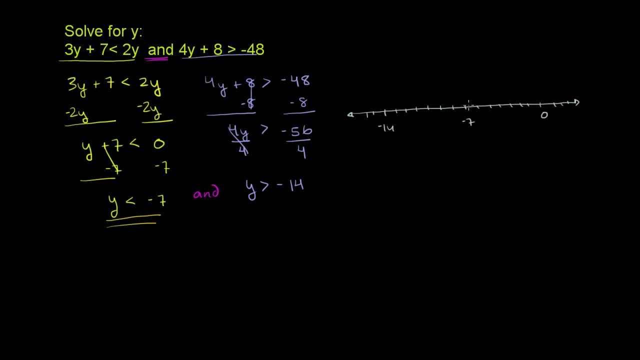 So let's look at this: Less than negative 7. So not including negative 7.. So we'll do an open circle around negative 7. And less than negative 7. And if that was the only constraint, we would keep going to the left. 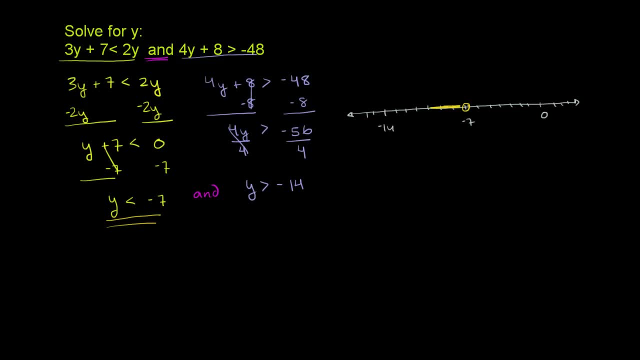 But we have this other constraint, And y has to be greater than negative 14. So you make a circle around negative 14, and everything that's greater than that, And if you didn't have this other constraint, you would keep going. 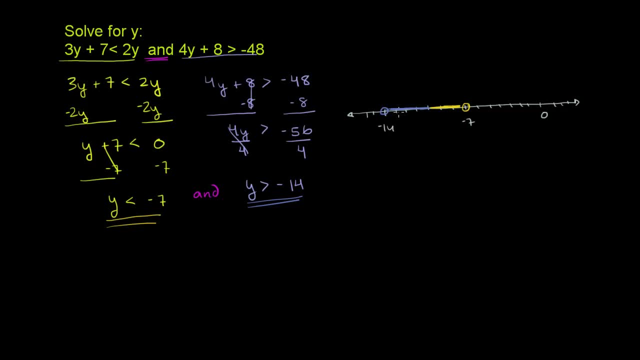 But the y's that satisfy both of them are all of the y's in between. These are the y's that are both less than negative 7 and greater than negative 14. And we can verify that things here work. So let's try some values out. 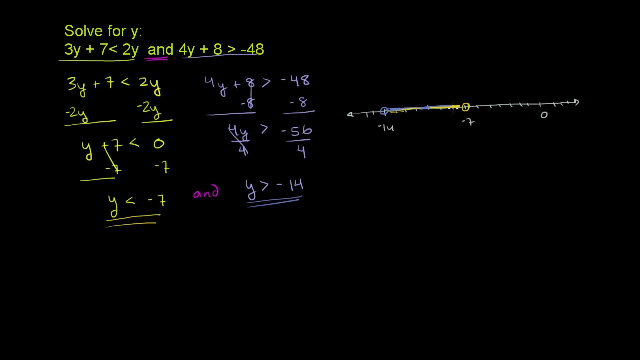 So a value that would work. well, let me just do: negative 10 is right here. 8,, 9,- this is negative 10.. That should work. So let's try it out. So we'd have 3 times negative 10.. 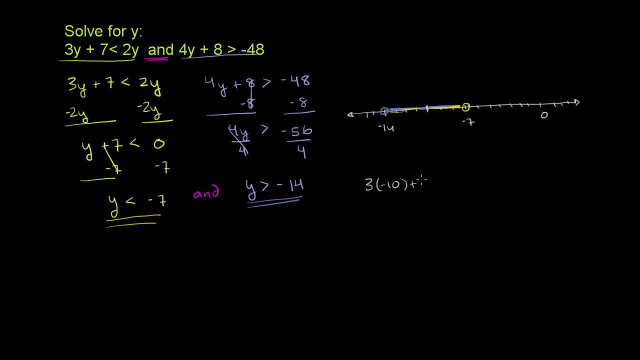 Negative 10.. 3 times negative 10 plus 7 should be less than 2 times negative 10.. So this is negative. 30 plus 7 is negative 23, which is indeed less than negative 20.. So that works. 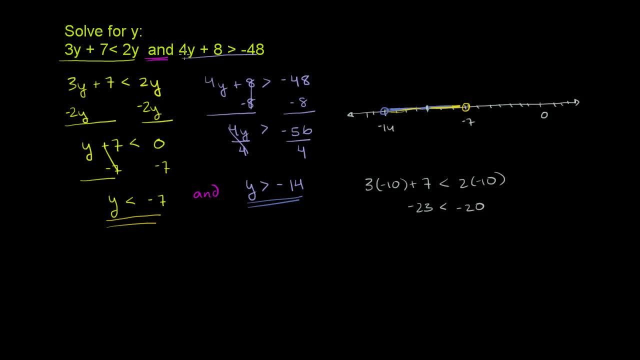 And negative 10 has to work for this one as well. So you have 4 times negative 10, which is negative 40, plus 8.. Negative 40 plus 8 should be greater than negative 48.. Well, negative 40 plus 8 is negative 30..